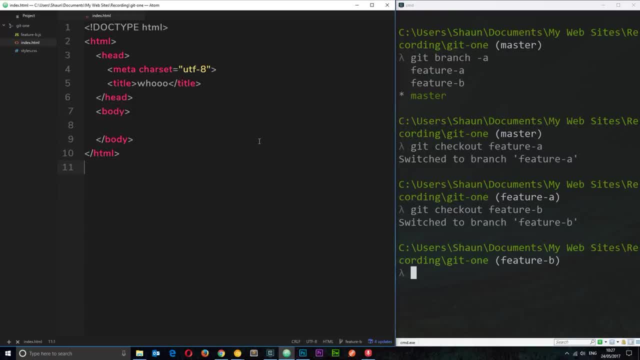 So to do that, first of all we have to be on the branch that we want to merge into. So we want to be on the master branch, because that's what we're merging into. So I'm going to say: git, checkout, master. 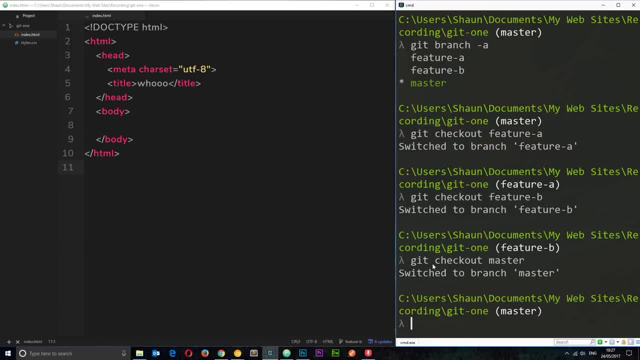 Okay, now what we want to do is merge that feature a branch into this one, and to do that we just say git merge, and then the name of the branch that we want to merge in, and it's called feature hyphen a: Okay, so now we see this message updating fast forward. 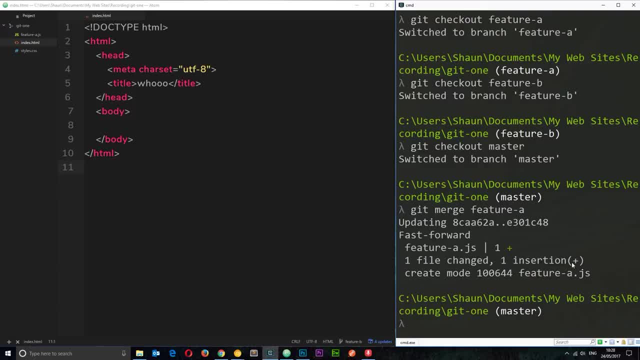 Feature ajavascript. one file changed, one insertion. Okay, so now what we've done is we've taken that code from the branch the feature one branch, or feature a branch, and we've merged it into this master branch, which we're still on. 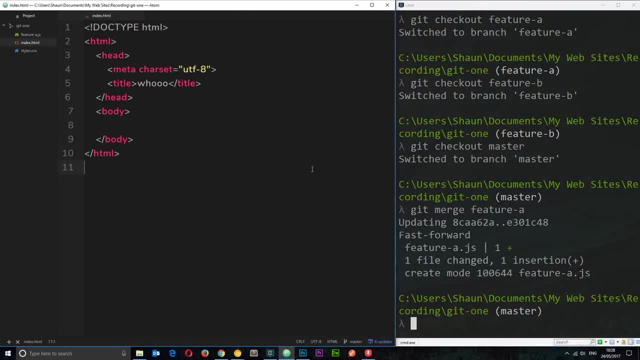 and now we can see that feature a script right there. So cool, we've merged that now And this fast forward thing basically means that all we're doing is kind of fast forwarding up to the code changes that we've made in the feature a branch, because in the time between branching out 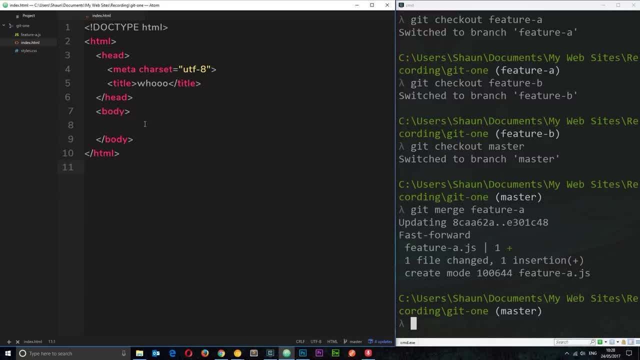 and merging it back. So we've not actually made any changes in the master branch. So essentially all we're doing is fast forwarding up to that feature. a change, Make sense, Cool. So now let's merge the other one. 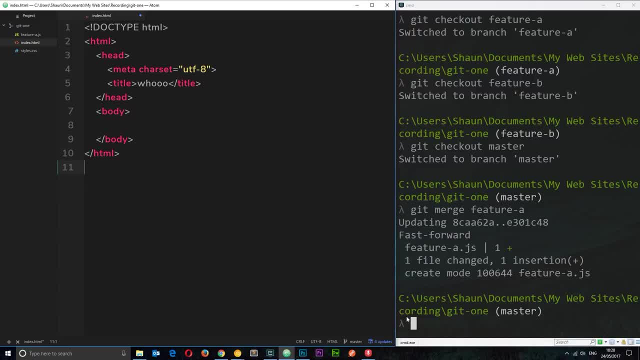 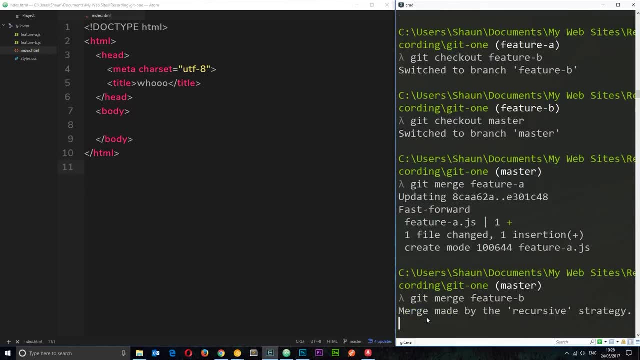 So we do the same thing. We say git, and we don't do it in the text editor, We do it over here: Git merge, and then we want to merge feature hyphen b. So let's do that, This time we merge feature b and we can see feature b over here as well. 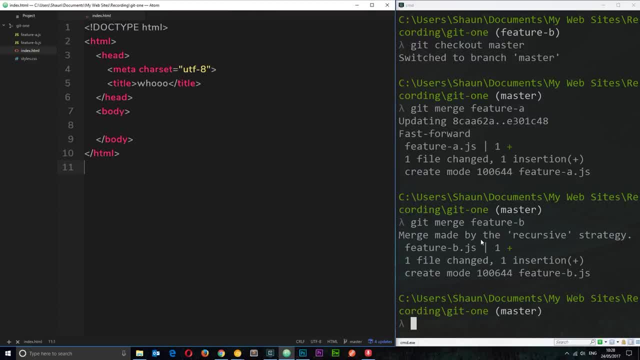 So that's worked successfully. The only difference is that this time The merge was made by the recursive strategy, And that's because this time we've not just fast forwarded to this branch code, because this branch code didn't have feature a in it. 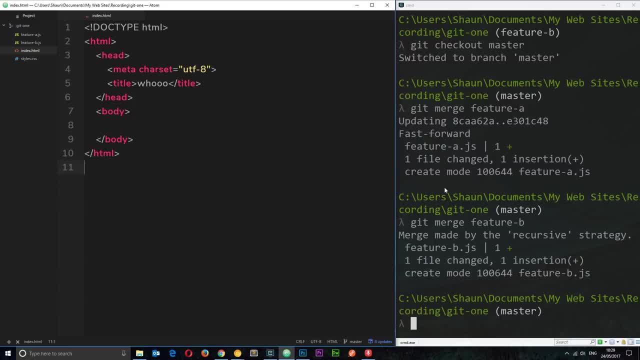 In other words, the master branch has changed in the time from taking feature b branch out and merging it back in because we've added the feature a branch to master. Okay, So it has to use a different strategy. to merge them Doesn't really matter so much, just yet. 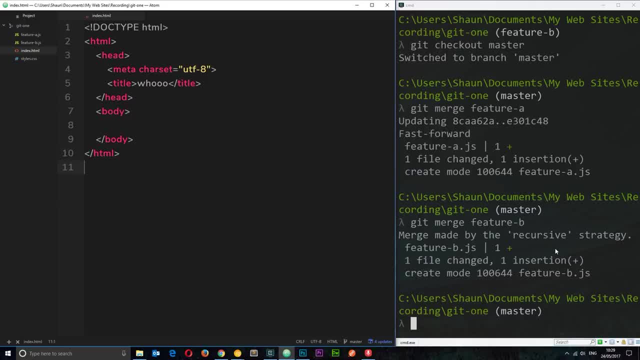 The same effect is here. We've still merged the feature Feature b branch into the master, So now master is up to date with both of these two features, And it doesn't matter that we've worked on them at the same time. 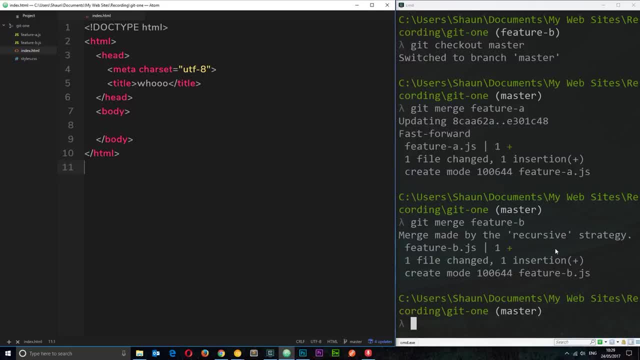 Different people doing them. We've both just merged them back in and everything is absolutely fine. Okay, But that's not always the case. Sometimes you're going to come across what's known as conflict, And I'm going to give you an example of that now. 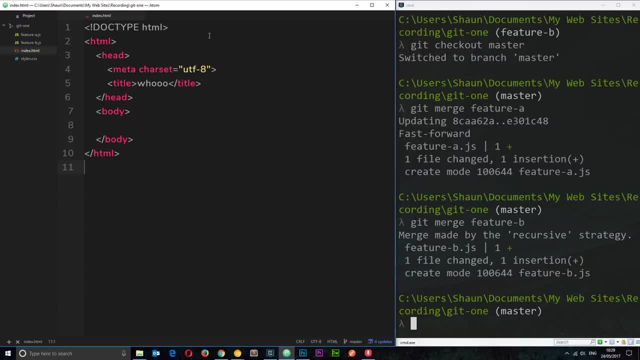 So, for example, Say: this is the current state of our master branch: Everything's happy, The code is working perfectly, And we want to add in a new feature, A new CSS feature- right, So let us check out a new branch to do that. 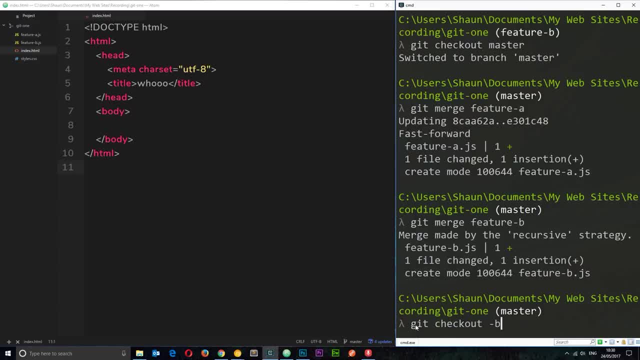 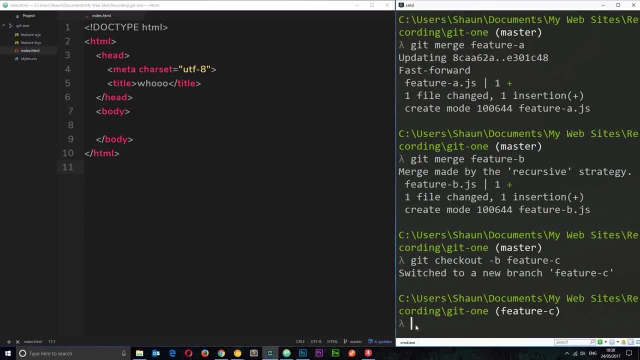 So I'm going to say: git checkout hyphen b to say we want a new branch And also the branch name which is going to be feature c. Yep, I'm terribly original, Okay. So now we're on this, feature c branch. 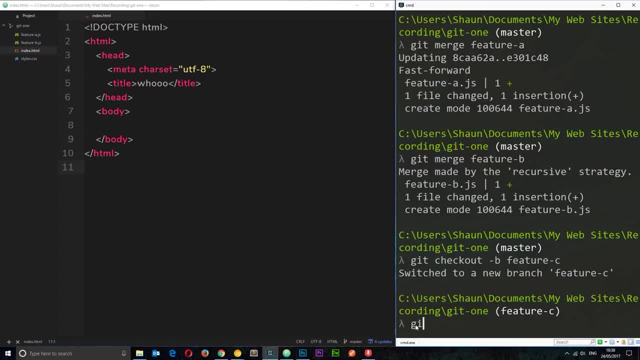 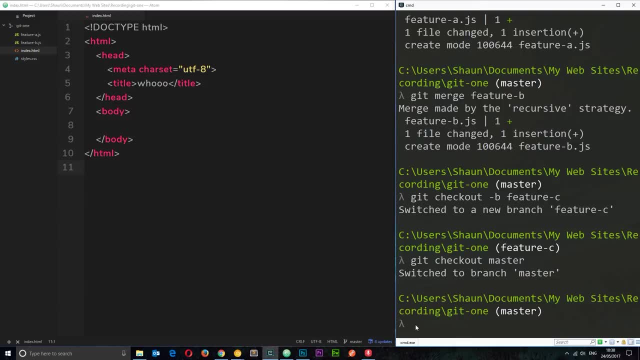 But before I start work on this, I just want to go back to the master. So I'm going to say: git, checkout, master. Now we're back on the master branch. Now I want you to imagine that some upstart new at the company has decided just to make edits on the master. 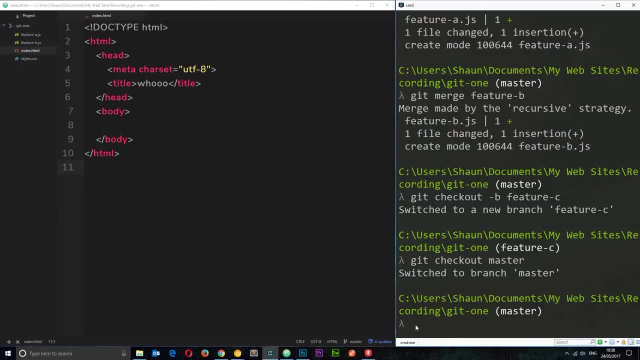 Yep, those people do exist. So what they've done is they've gone into the CSS file and said: you know what? I think I'm going to put a margin of 20 pixels on this body selector right here. Okay, So I'm going to save that now. 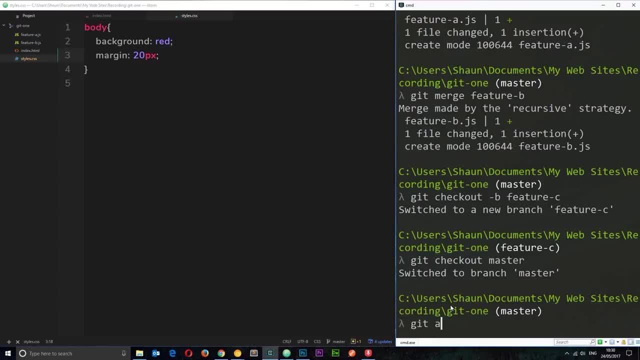 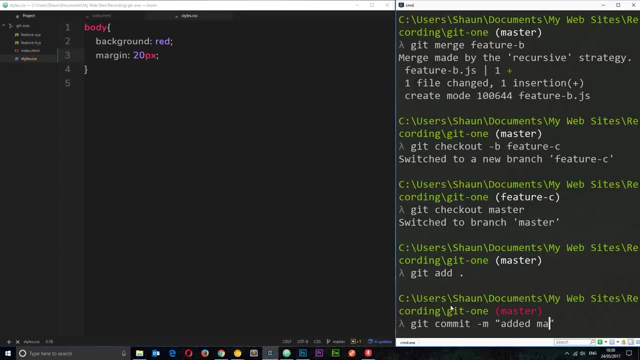 And I'm going to commit it to the master branch. So let's say git add, just to add those to the staging area. Then we'll say git commit And the message is added. margin to the body selector. All right, Cool. 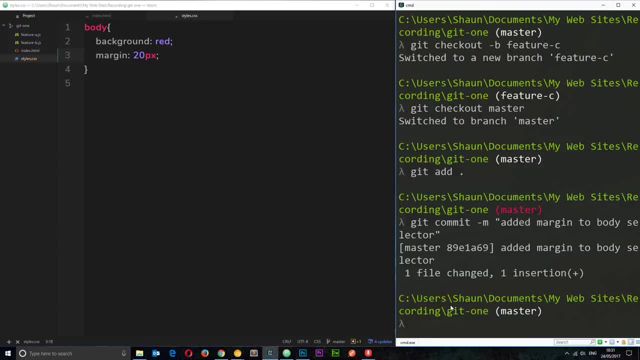 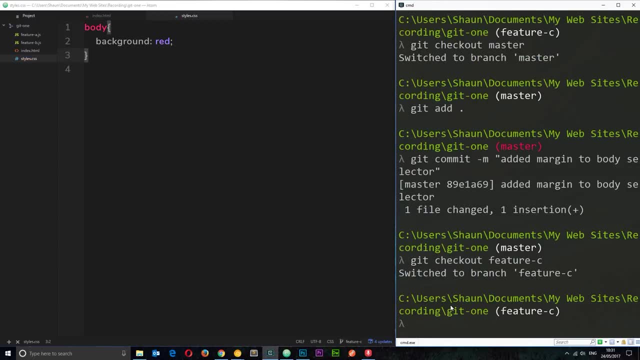 So we've made that commit now. Now, in the meantime I'm working on feature c, So git checkout feature hyphen c. I'm working on this And I don't know about that CSS change that the other dudes added into the master branch. 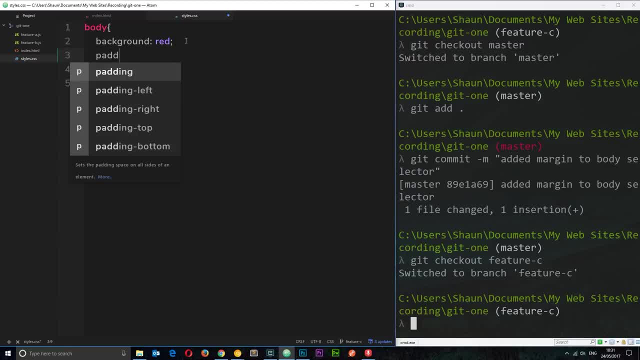 All the time I'm working in the CSS file and I add in a padding property to the selector, which is going to be, I don't know, 30 pixels, right, So I save that. now. I'm happy with this new CSS feature, which is really cool. 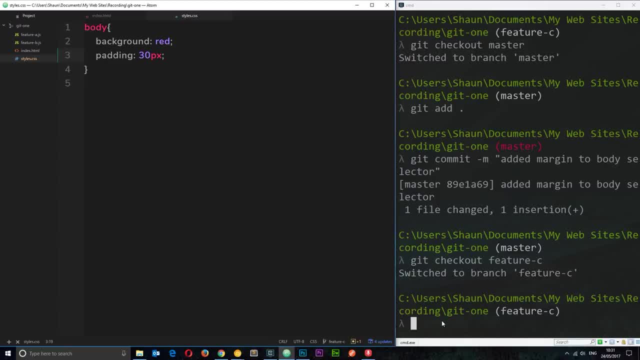 And what I want to do is merge this. So I'm going to merge this back into the master. So first of all, we need to make a commit to this branch. We'll say git add to add these changes to the staging. 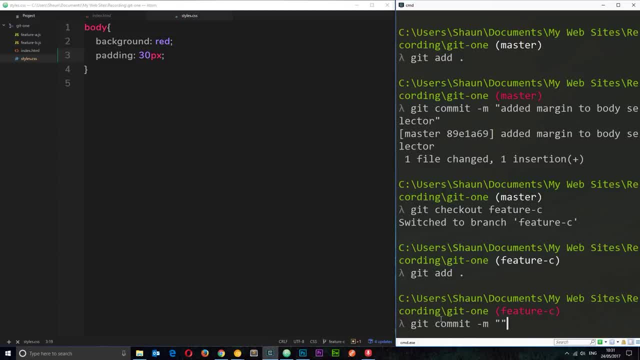 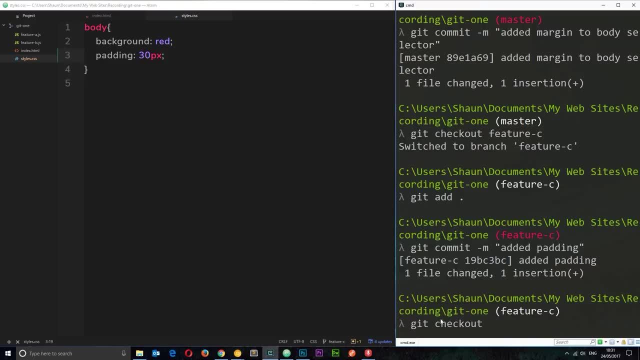 Then we'll say git, commit, and m is going to be added padding. Okay, That'll do. Anyway, now I want to merge this, So I'm going to check out the master first of all, because that's what we're merging to. 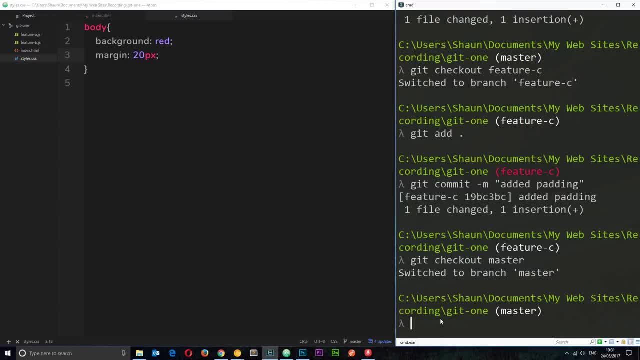 And now I want to merge the feature c branch into master. So what I'm going to do is say git, merge, And then the name of the branch, which is feature c. Now check this out. Boom, We have a conflict, right. 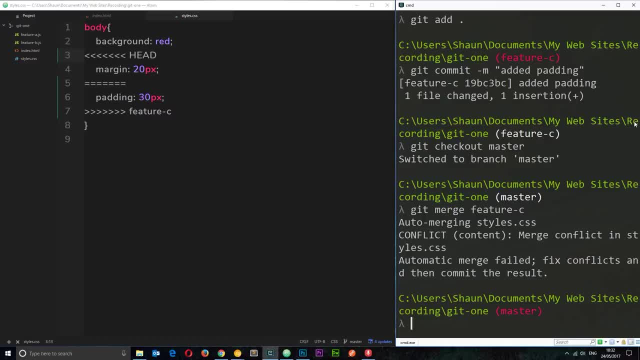 And that's because that upstart has been editing the body selector in the master branch while I've been working on my new feature editing the same selector right, The body selector. So in this case we get a load of mumbo jumbo over here and we also get an error message. 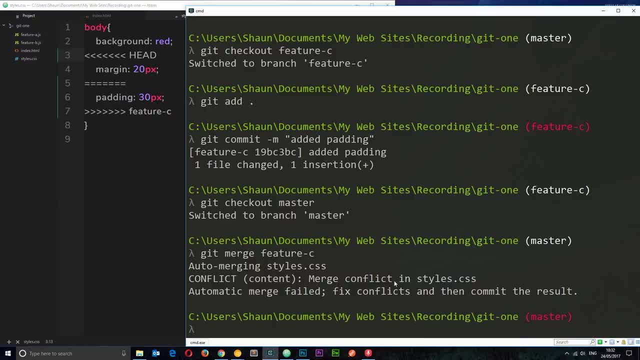 over here An error message basically says: there's a conflict in the stylescss file. That's nice. It tells you which file it's in. There's an automatic merge failure. There's an automatic merge fail And it tells us to fix the conflict and then commit the result. 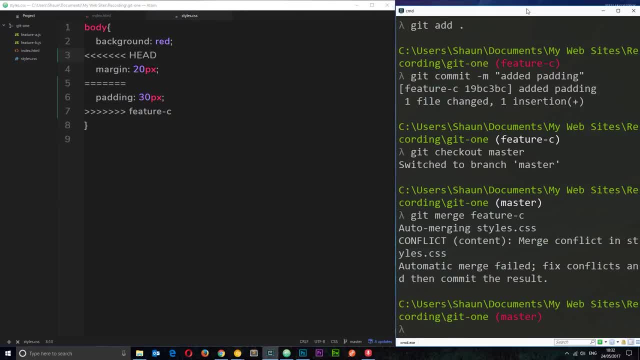 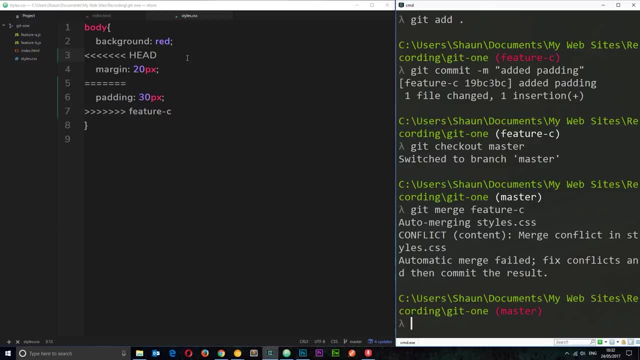 So it's asking us for help because it doesn't really know what to do at the minute. It's a bit stuck because it knows that someone's changed this select on the master branch and someone's changed it on this new feature branch. We're trying to merge the two together and git doesn't really know which version we want. 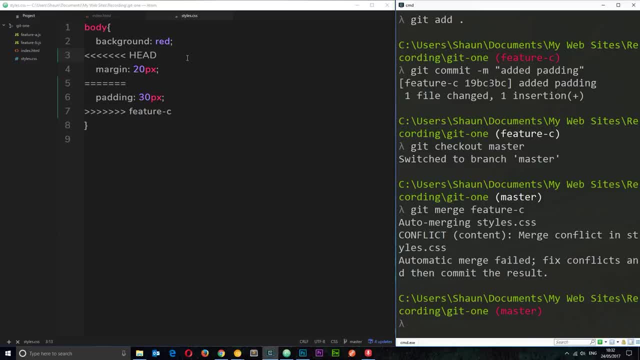 okay. So we have to help it decide. So all we want to do basically is say: to git what we want in this code. Now I've had a you know, speak to this new guy and said, okay, don't develop on the. 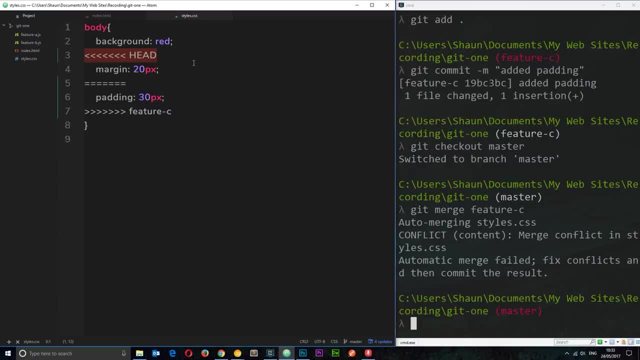 master branch again. but what is it you want? And he says, yeah, we do need that margin there. So I'll keep the margin in. I'm going to delete this little comment thing right here and this thing right here, And also I want to keep in the padding. 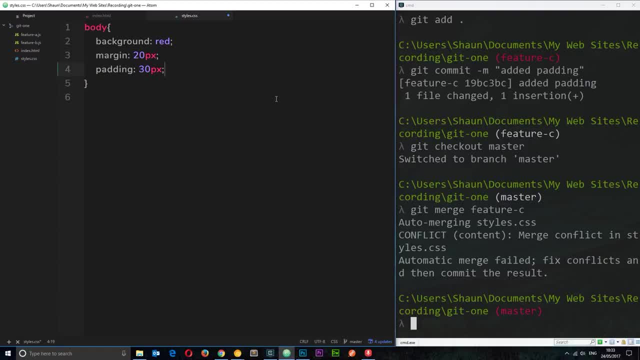 So we'll delete that, but leave everything else the same. So this is basically how this body selector should look, right? So now, if I save this, what I'm going to do is add this file. I'm going to say git: add to the staging area. 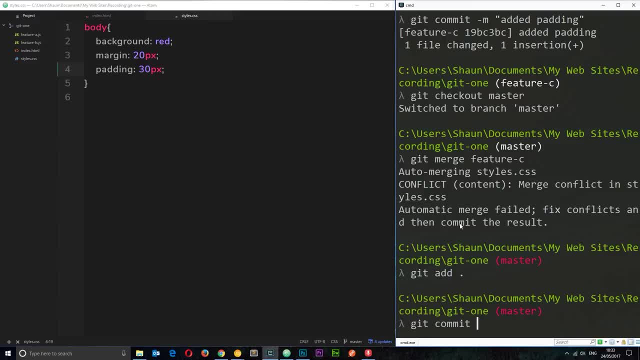 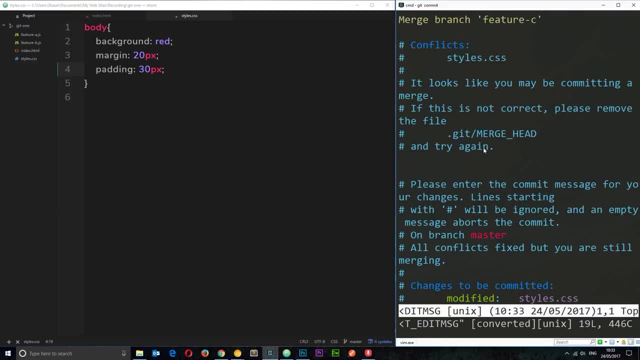 Then just do a git commit. Now, this time I don't need to write a message, because we're just doing like a kind of merge commit, if you like. So I'm going to just say git commit and then you'll get this scary screen again. 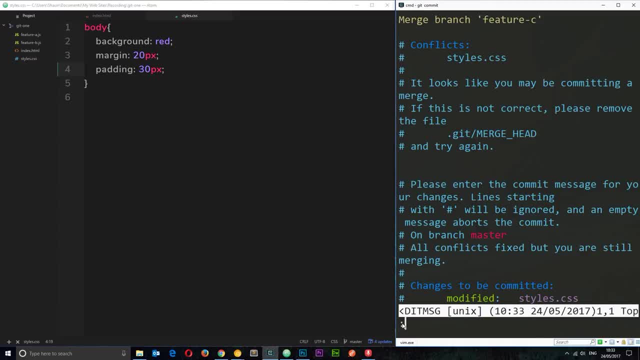 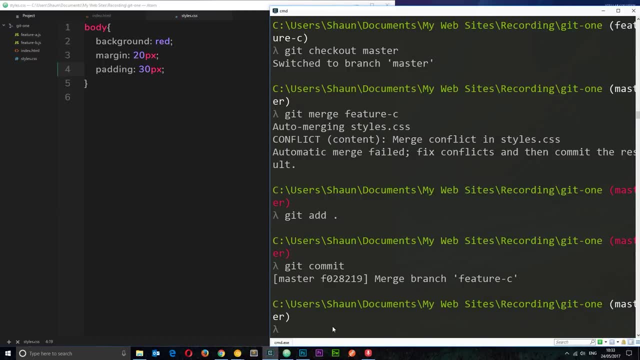 You don't need to do anything except shift and colon. You'll see this colon down here now. Then wq enter, It's going to exit out and it's going to do that merge for us. So now everything is hunky-dory.